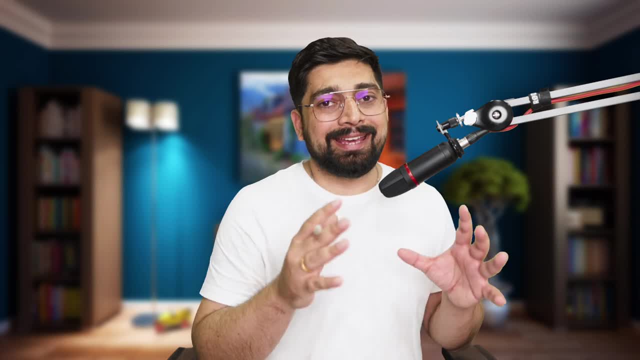 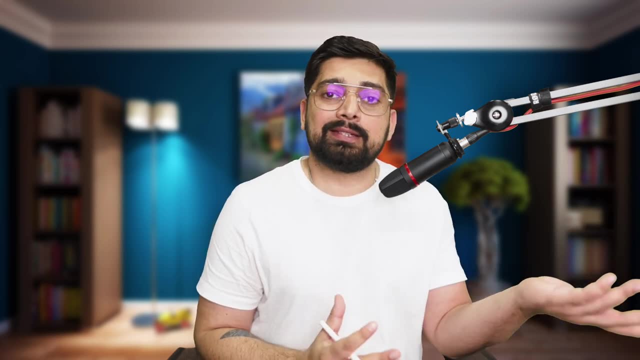 is whoever bears that token. whoever holds that token is a valid user and I would allow them to authenticate in my application. Now, in case somebody steals that token, then he's the bearer and he is totally allowed. Now, this small sentence actually gives a lot of anxiety. 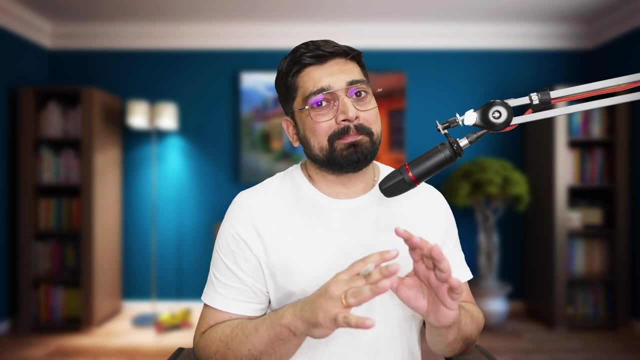 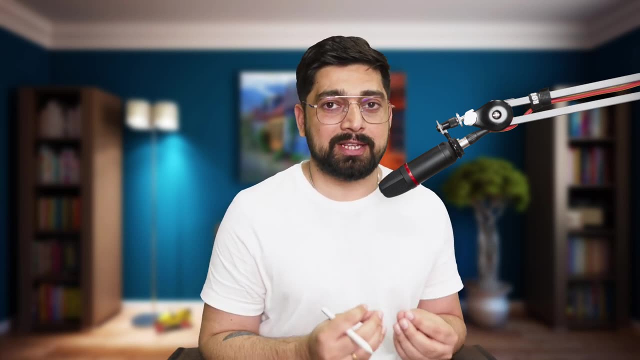 to a lot of people that. is it even a secure mechanism? Now, in my actual run through of the building a lot of application, JWT is pretty good and solid resource to authenticate a user. There is nothing to be worried about, In case you are a little bit worried. 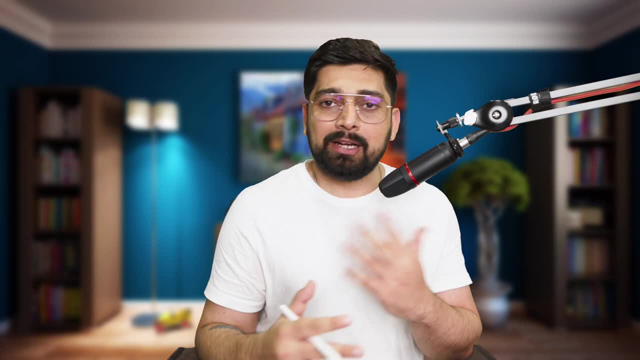 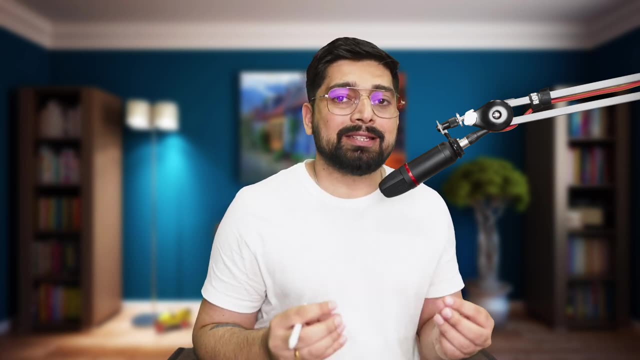 you can additionally use a concept of refresh token, But I'll talk about separately in another video about a refresh token, because it's not a mechanism to secure the token, but rather a mechanism so that user doesn't have to log in again and again. So we'll talk about them later on. 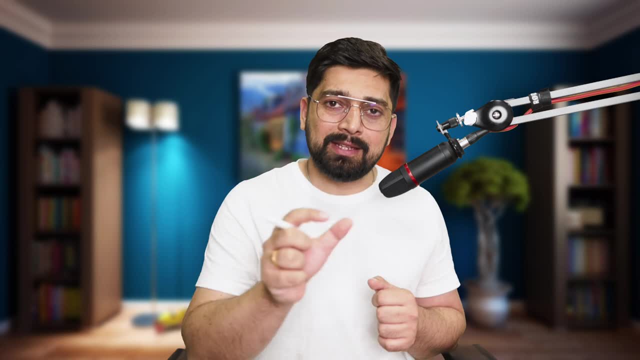 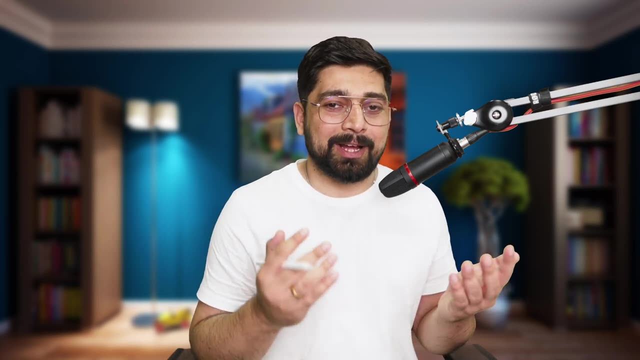 So, again, both of these techniques are just to make sure that we give something to the user so that we can authenticate them later on and keep on authenticating them without having to allow them to set the password in every single refresh page. So that's what it is. 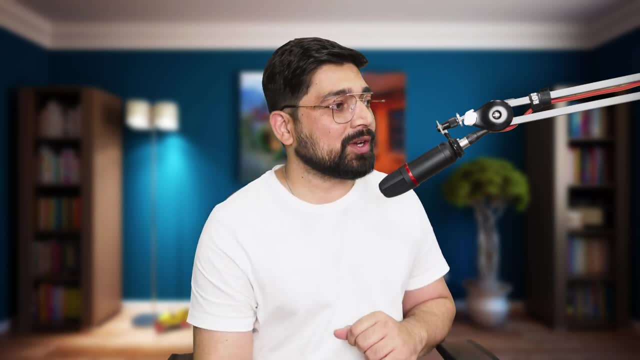 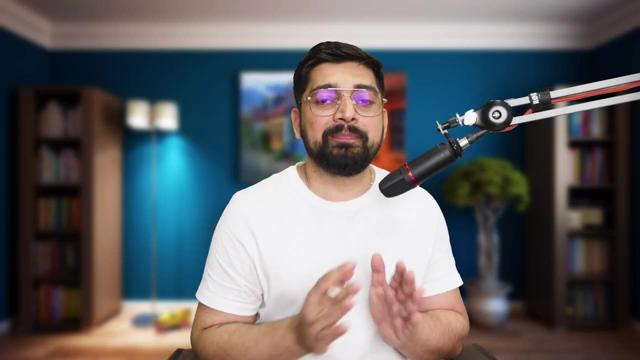 Now a lot of time. people have a discussion on this And, by the way, in case you are worried, don't be, I do have my notes here. We'll talk about the refresh tokens and JWT tokens in just a minute. First of all, this is entirely related to the back end. 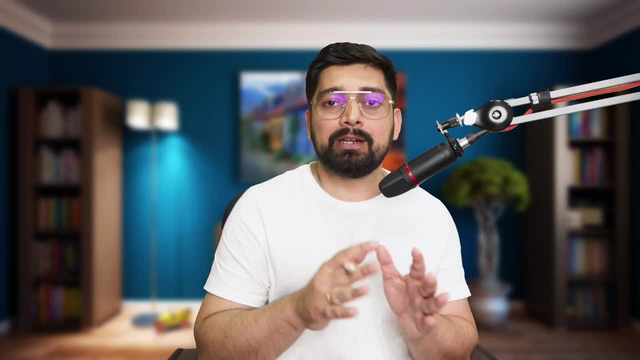 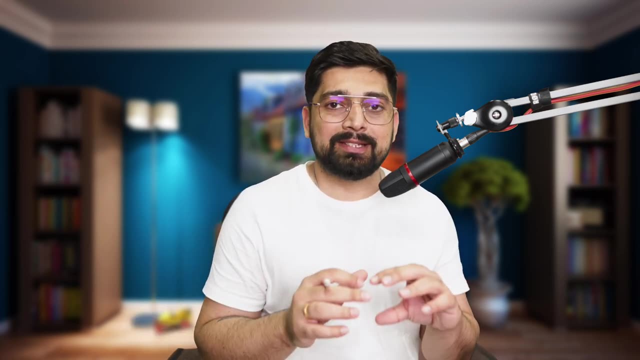 So all those people who don't actually are able to understand this, just remember this is a back end technique. When you will learn authentication in the back end side, this is something that you'll be using. So JWT is a mechanism which is quite popular. 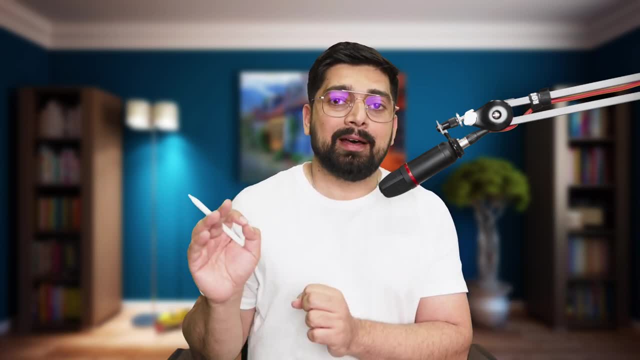 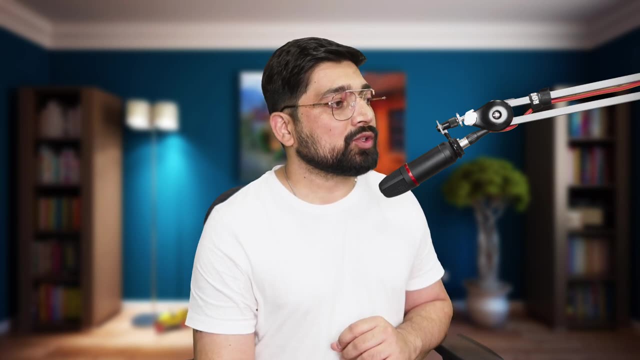 and is being used, but still some of the people prefer to have the web server token. So I'll talk about them as well, how they are useful and how even they are actually being designed in a minute, But first let me walk you through to all those people. 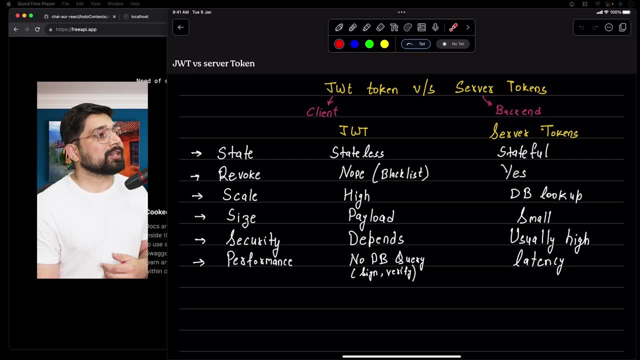 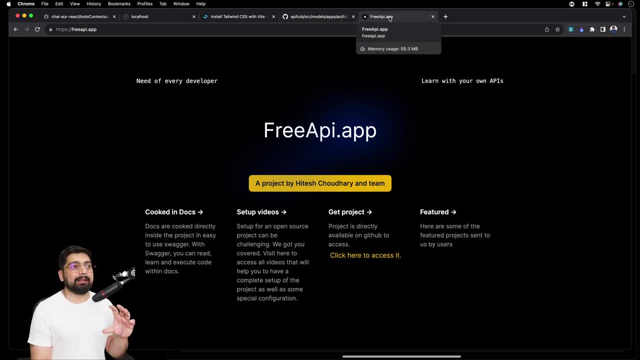 who probably don't like to watch that much of video and still want to explore the things. So let me first go back here And what you can do is you can go to free API And if you want to understand the mechanism of how the refresh token and all these things works, 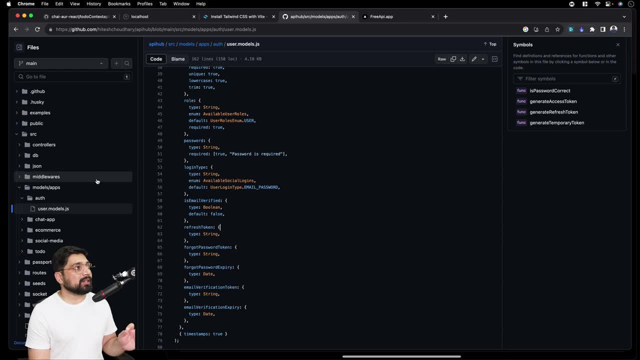 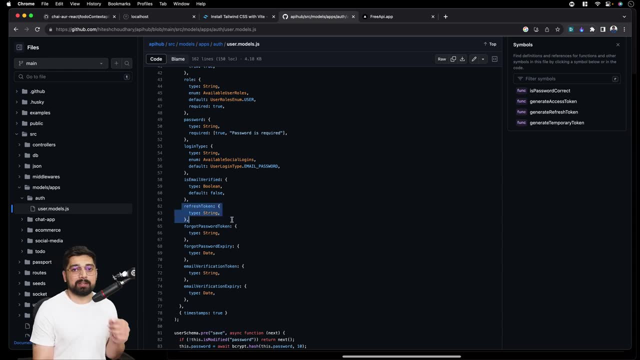 just click up here. This is an open source project And you will notice here that inside this project, inside the source, if you'll check out the models, we are actually holding these refresh tokens in our servers Later on how the mechanism of refresh token works. 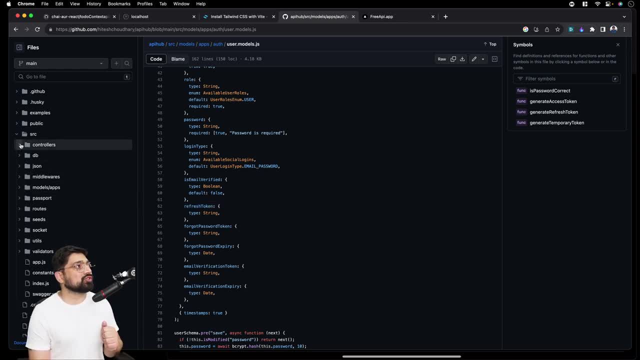 you can actually just study them directly by going into the controllers, And obviously this is something that we used in the apps for logins. So there is an auth app. you can just click on this And in the user controller, everything is mentioned here. 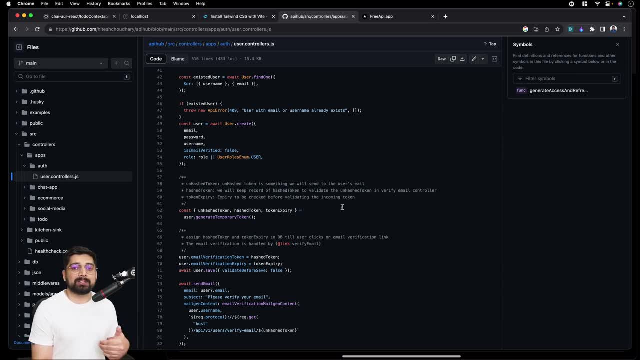 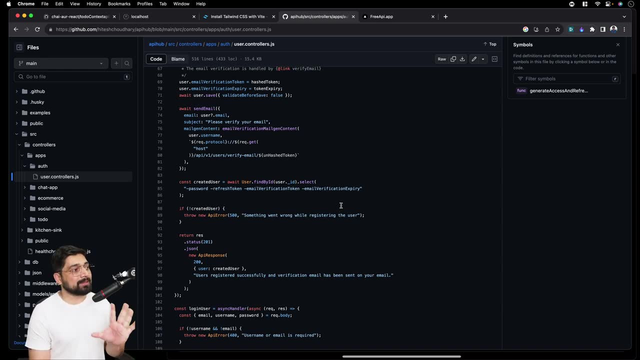 So you can just read the study, the code, and probably will be able to understand all these things much more faster that how the refresh token mechanism works, when we are updating them, when we are making a query about them. That's the basics of it. 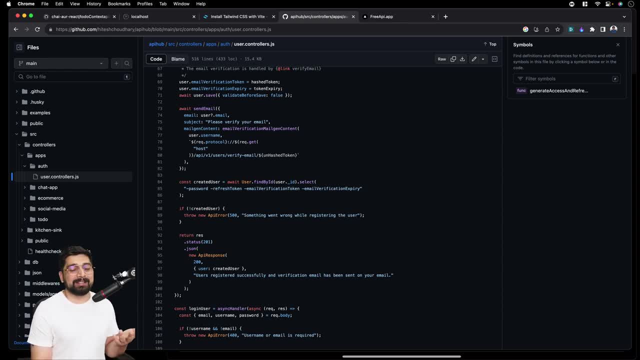 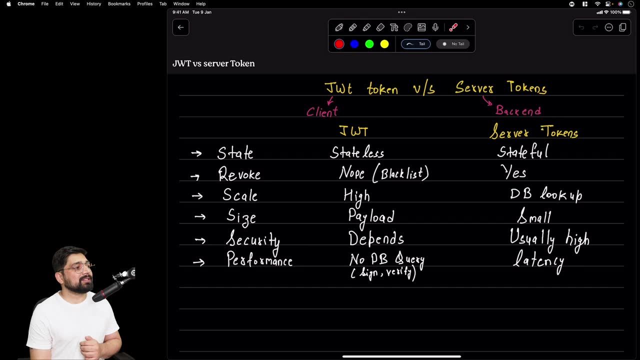 in case you want to go into the code, part of it I'll obviously create. we'll be creating more videos on that, but that probably will be on another day. Now let's come back on to this part. So this is something that we are going to discuss. 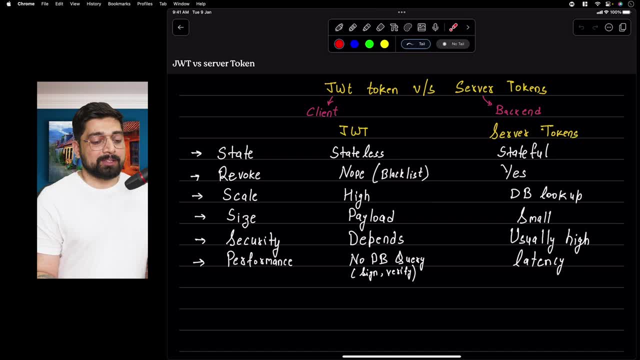 about the tokens and all these mechanism that goes through. So, first of all, let's talk about: this is the part where we actually go with the JWT tokens, And this is the part where we go with the server tokens. Now, JWT tokens are actually, moreover, the client tokens. 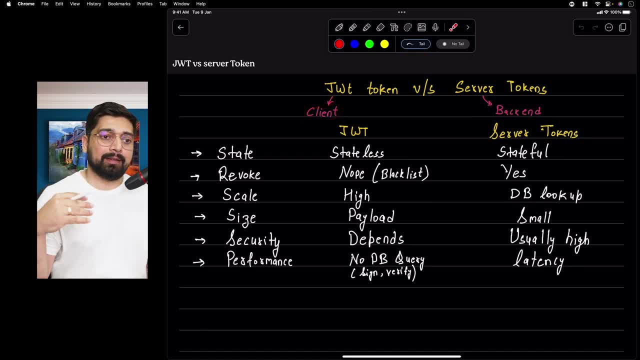 So they are given to the client Once you generate them. in the backend. there are packages for generating the JWT tokens. It is actually being built up of three major parts. The more important one is the payload part, in which you can add some information. 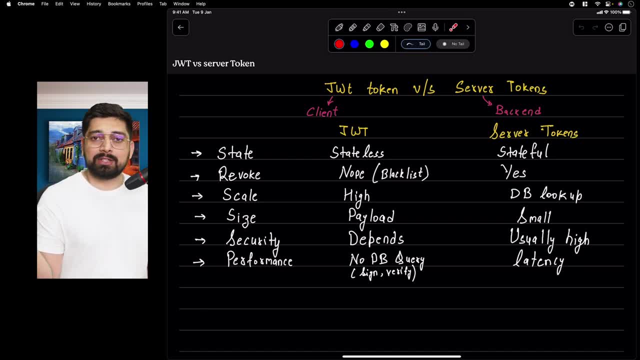 It could be just an ID of the user, so that later on you can make a backend request and find more information. Or maybe there could be a username, a profile picture, URL, whatever you want to inject, that's a payload, you can inject that. 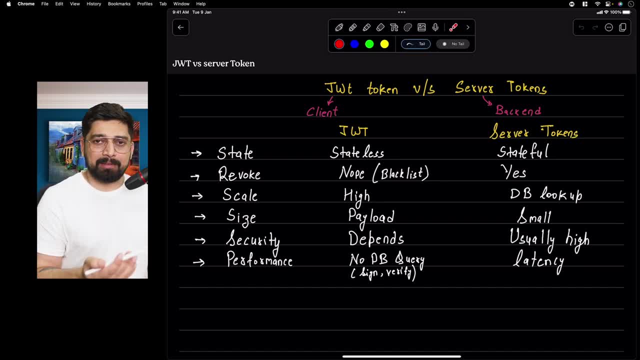 And that is being sent to the client so that whenever we need to verify that are you a valid user or what, so username or anything that's there in the payload- we can actually get that. That is given to the client and client. it's up to the client how it stores them. 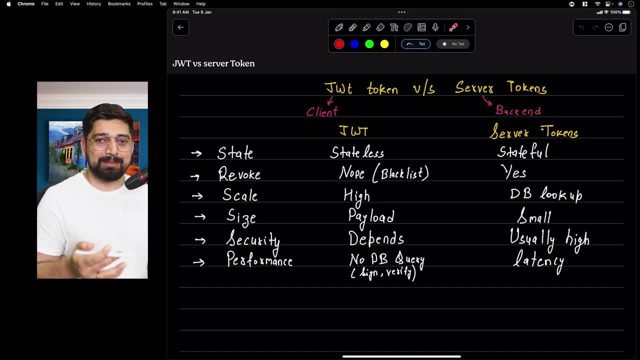 There are obviously great ways, bad ways. So there's: some people store them in the cookies- secure server cookies. some people store them into the local storage. Maybe there's a different case for each one of them. let's not judge them directly. 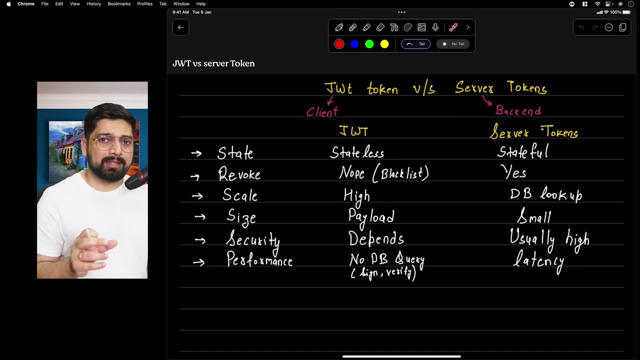 And there are also server tokens. They are also kind of a similar in look as we see that the JWT tokens, but they are just a random string generated by I don't know what resource, maybe crypto, or however. you are generating them. Once you generate them, 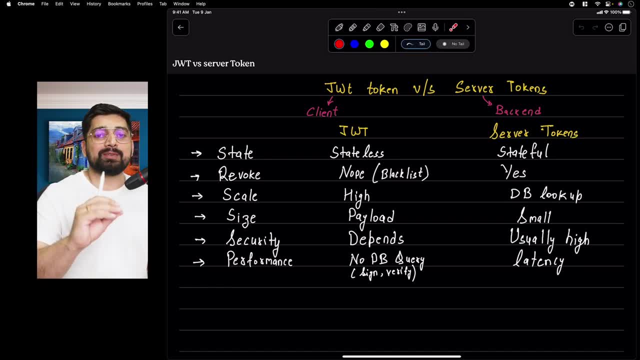 you actually store them on your server as well, like in database, as well as you send them to the client as well. So the only difference is that we store some things in the server and sometimes we don't store anything. we just send it to the client. 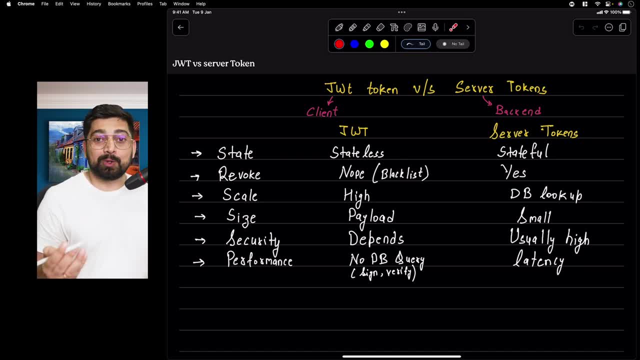 So that's the whole idea about the JWT token: that it's a bearer token. Whoever holds that token is an authorized user. And yes, there is an expiration time that you can set up If you're worried about it, that I don't want to set too long of an expiration time. 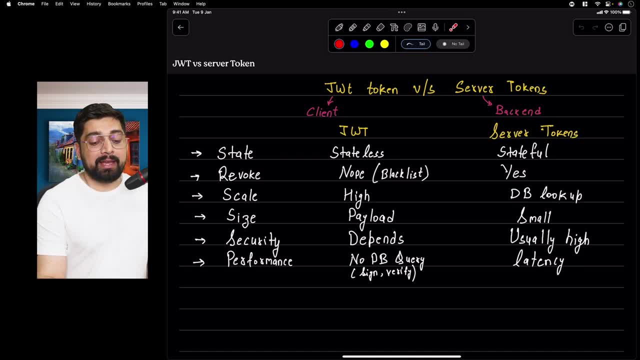 or I'm worried about it. that's where the refresh token concept comes in In the server tokens. we just store them since on the server and is being given on to the front end client as well. We all the time make a query on the backend. 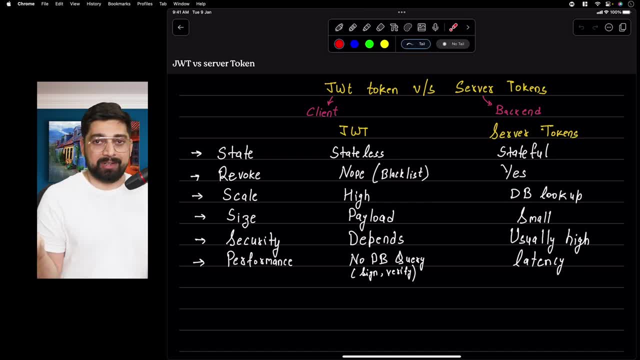 to verify that. does this token match? It's almost like a password, but not really password. So, in case you want to understand more about them or can have a conversation on that, there should be some parameter on which we can actually have this conversation. 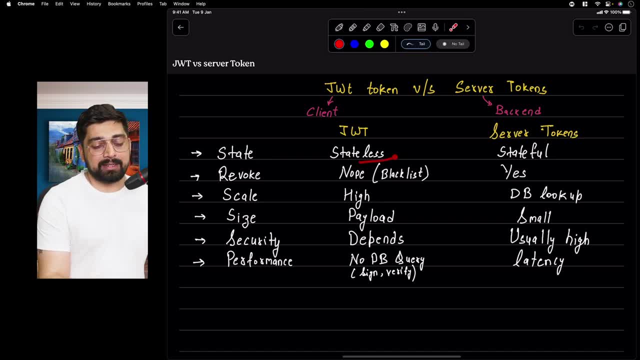 The first one is the state. So the JWT are considered as stateless, while the server tokens are considered as stateful. The whole idea is just the same. Stateless means whoever holds them is the owner of it. Yes, there could be more discussion. can happen that. 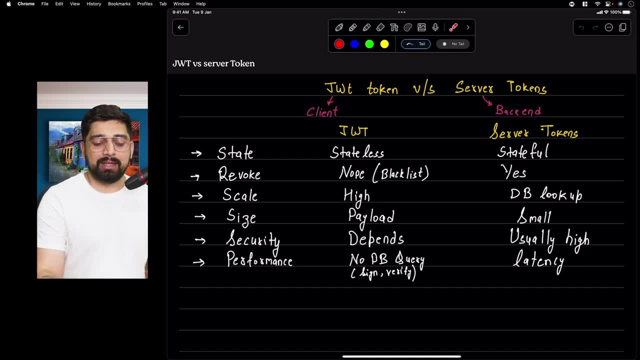 but, in general, just keep in mind that JWT tokens are stateless token and the server tokens are, moreover, a stateful token. Revoke access. can I revoke them? Sadly, there is no mechanism of revoking the JWT. Once it's given, that's it, it's given. 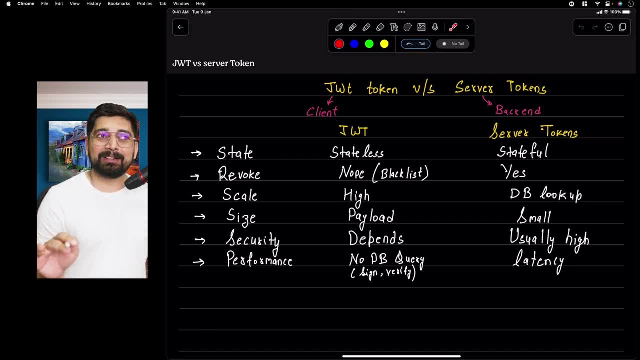 Until unless there is also a mechanism of or a strategy that you can have a list of blacklist tokens and once you add any token into the blacklist, that's it. he cannot just log in. But again, most of the time you'll just say: 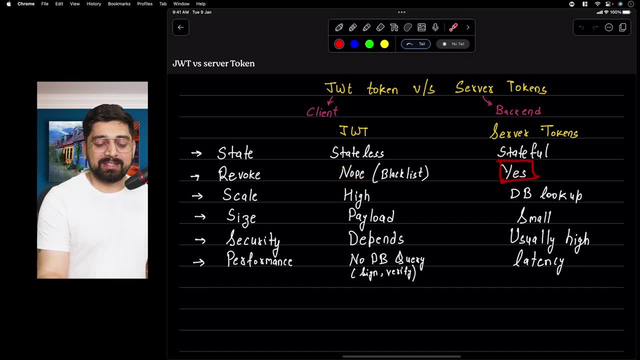 hey, there is no way to revoke the JWT tokens For the server tokens, since everything is being stored in the server. that's it. You can just revoke all the tokens and just log out forcefully every single user. The scalability is an issue. 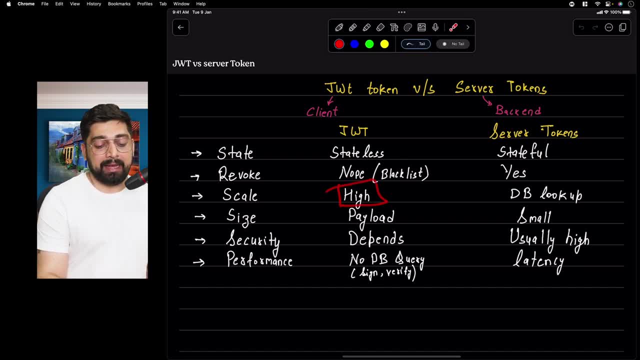 which you should really consider because the scalability is high And in this one, whenever you actually store tokens on server, you always have to perform a database lookup. So the more database lookup, more database query. that means scalability can be a question here. 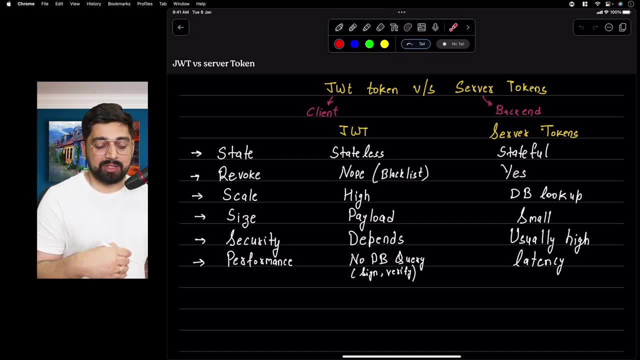 And in case of JWT, since you are just generating them, you're just saying them that, hey, this is all done and gone. But remember, when you generate the JWT tokens, there is a compute time that you have to be worried about. 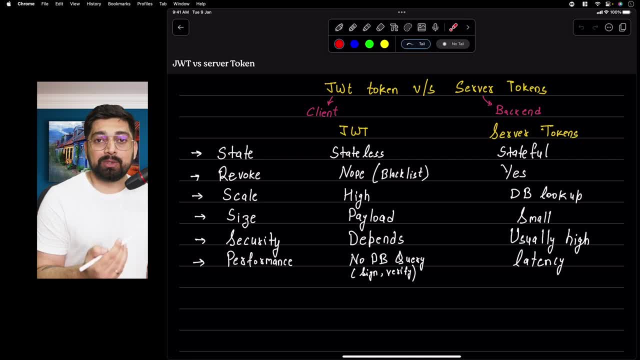 And that's why we most of the time use await keyword in front of JWT, because it's a compute heavy thing And it takes a couple of milliseconds. so you need to use await in case you're using JavaScript there In case of the DB lookup, just be worried. 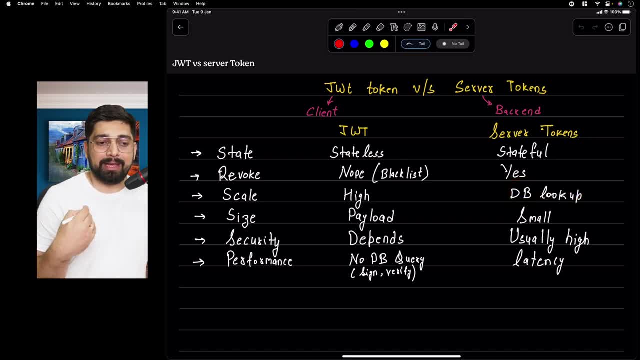 if you're storing everything in the server, just like you, every time query images, URL or maybe something else. Similarly, you have to query: for every single request, Every single page, you have to make a DB query. So the scalability is a big, big challenge in that case. 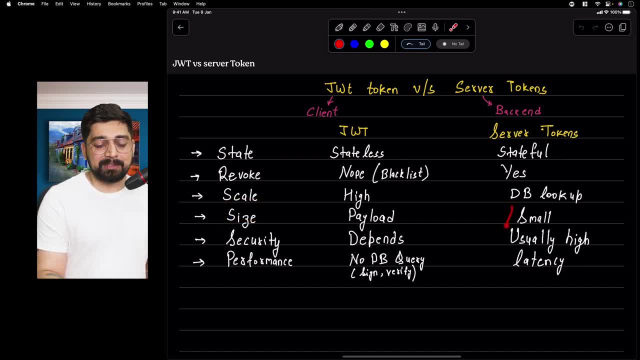 The size now- size of the something that you're storing in the backend- is relatively small because it's just a backend string, But in this case it's up to the payload. So in the payload maybe you're just injecting underscore ID. 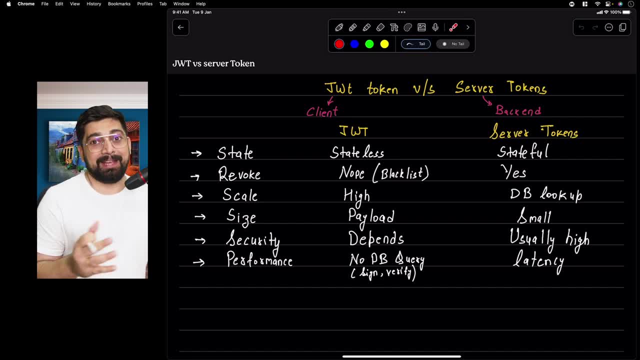 That's it. That's a very small one, But in case you are using something more, then, hey, this could be really really big one here as well. So size is very, very dependent on what you're injecting in the payload or what you're saving in the database. 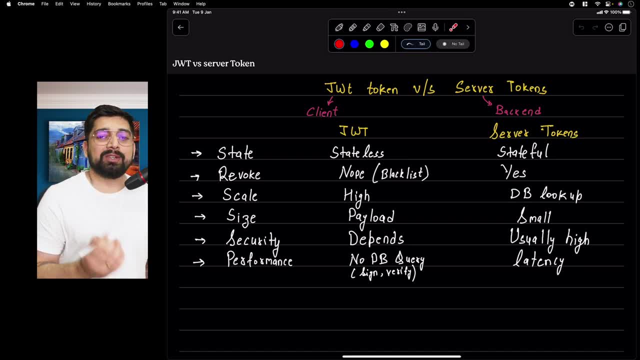 Now security. This is a big question here that: are JWT 100% secure? Over the years I've realized that there is nothing which can be called as 100% secure. but JWT are fairly, fairly secure. There are not too much of incident. 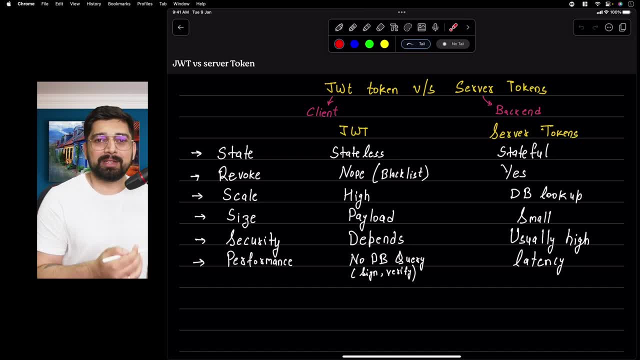 where people are just actually stealing your tokens And most of the time they are being stored in cookies which can only be manipulated by the backend only. So in that case fairly secure, But again it could be compromised Similarly if you just look at the backend tokens as well. 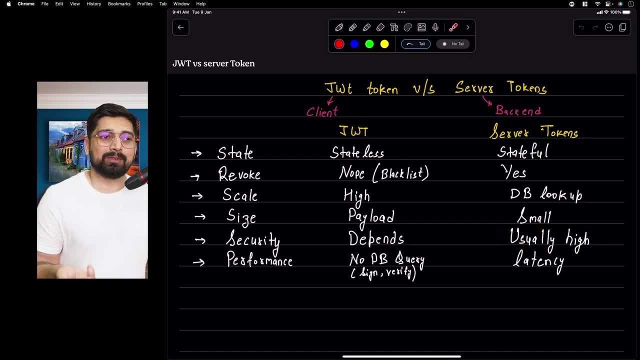 if somebody can steal the token given to you, he also can compromise your security. Now you're matching, It's almost like that. hey, I stole your password, So whoever has the password is the owner. So same concept actually is being worked.